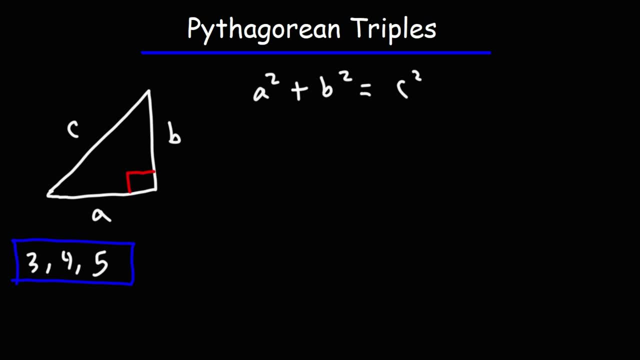 So this is the Pythagorean triple. This is the first one you need to be familiar with. The next Pythagorean triple is 5, 12, 13.. And you could test it in this formula: 5 squared plus 12 squared is 13 squared. 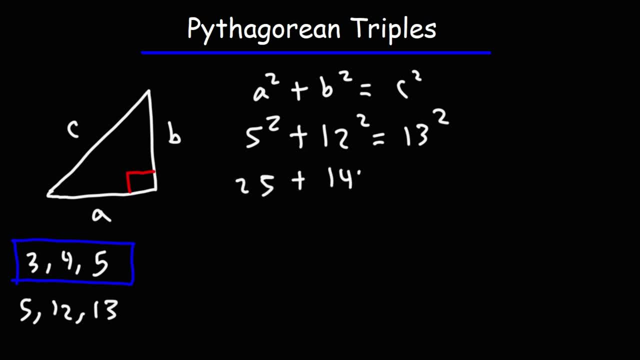 5 times 5 is 25.. 12 times 12 is 144.. 13 times 13 is 169.. Now 25 plus 144. That's 169.. So you can see that works as well. And of course the multiples of this Pythagorean triple will apply as well. 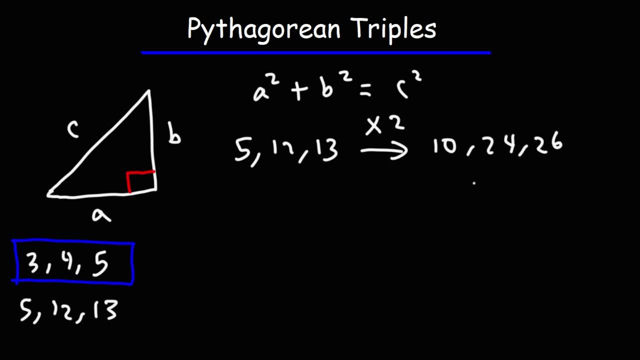 So we also have the 10,, 24,, 26 right triangle, The 15,, 36,, 39 right triangle, and so forth. But now, from here on, let's focus on just the base Pythagorean theorem, So the smallest, most common one which we've covered. 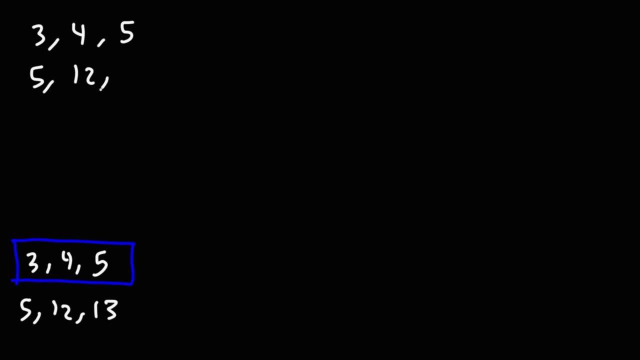 is the 3,, 4,, 5 right triangle. Next we have the 5,, 12,, 13 triangle. After that, the next common one that you'll see in school is the 7,, 24,, 25 right triangle. 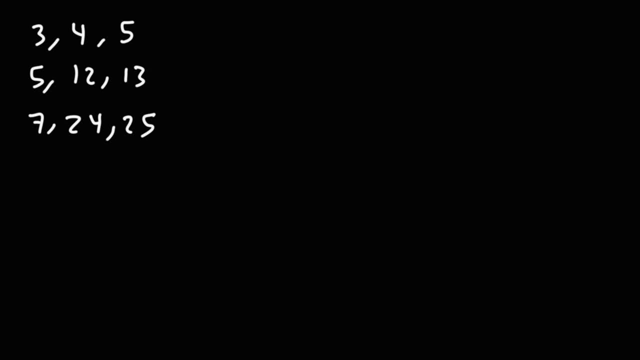 And then there's the 8,, 15, 17 right triangle. So these four are the most common base Pythagorean triples that you're going to see in a typical high school or college math course. Now there's some other less common Pythagorean triples. 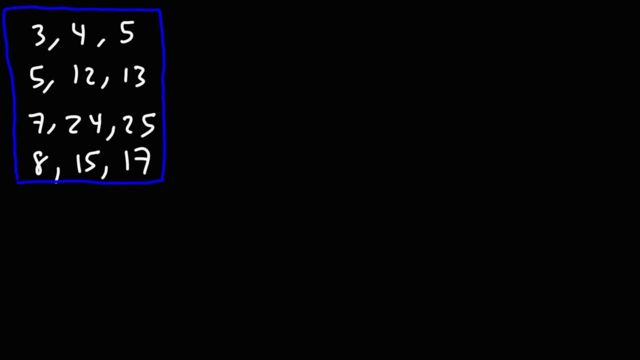 but you're going to encounter some of these as well. The next four is the 9,, 40, 41 triangle, And you could check it If you type in your calculator: 9 squared plus 40 squared, 9 squared is 81.. 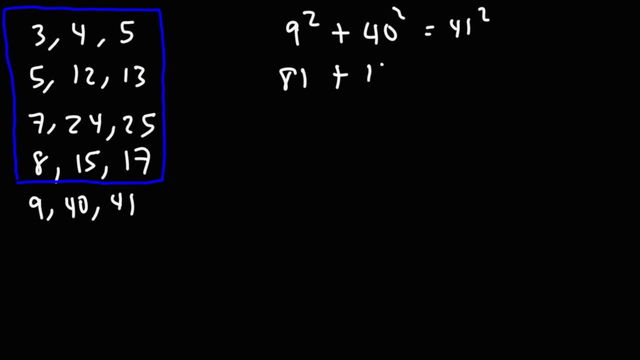 40 squared, 40 times 40, that's 1600.. And if you type in 41 squared, you'll get 1681.. So you could see that this particular Pythagorean triple checks out After the 9,, 40,, 41 triangle. 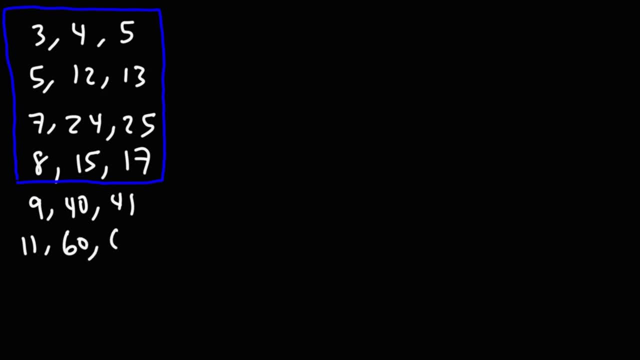 the next one is the 11,, 60,, 61 right triangle. After that it's the 12,, 35,, 37 right triangle, And there's also the 20,, 21,, 25, right triangle. So for these. you're typically not expected to memorize these, but I've seen them. 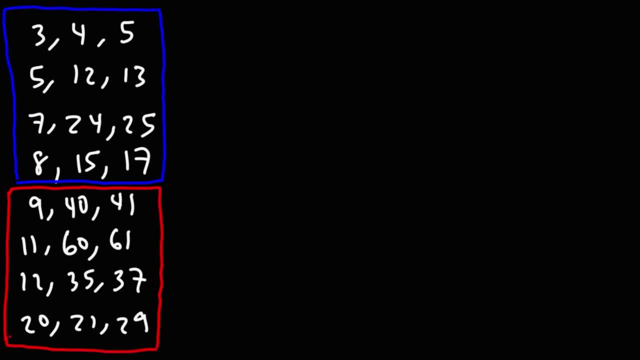 in certain problems, so you can add these to your list. So those are the most common Pythagorean triples that you're going to encounter in school. Now there's a lot more that are very uncommon. You really don't have to memorize these, but for those of you who are 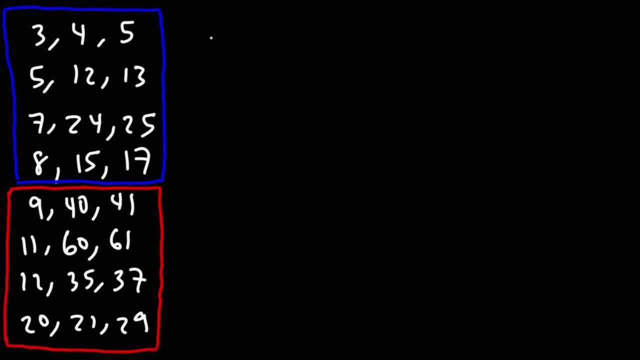 curious. I'm going to write them down. So the next one, the next few that I'm going to write are the ones that are under 100.. So we have the 13,, 84,, 85 right triangle. Next is the 16,. 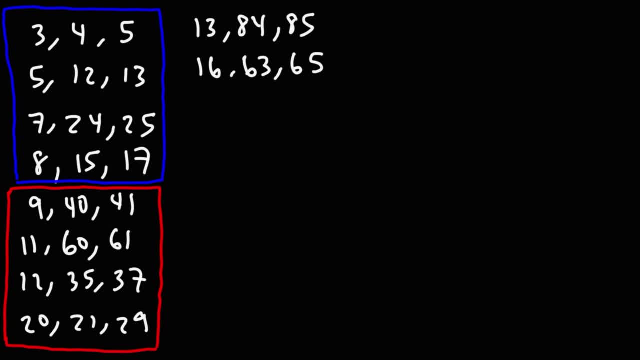 63, 65 right triangle. After that we have the 28,, 45,, 53 right triangle, And then there's the 33,, 56, 65 right triangle. Next is 36,, 77,, 85.. Then there's the 39,, 80,, 89.. 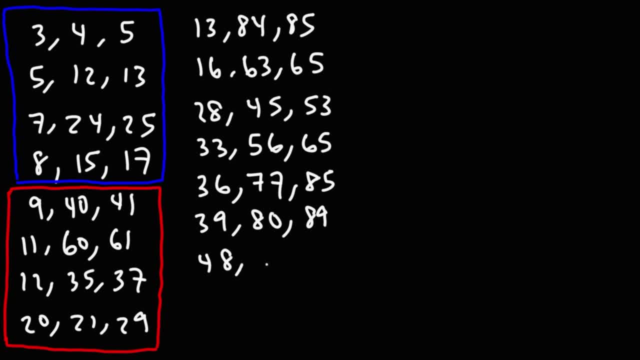 The 48, 55., The 43,, 73. And then the 65,, 72,, 97. And you could find these numbers online if you do a Google search. Just type in. you know a list of Pythagorean triples and there are websites. 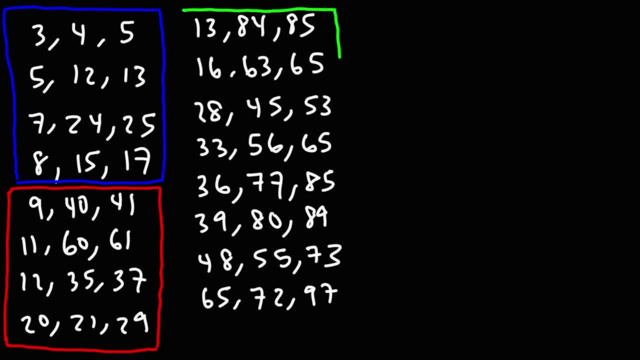 out there that will give you this, But for the most part you really don't need to know the ones highlighted in green. I've never seen them in a problem. The first eight, the ones highlighted in blue. you should definitely memorize those. The one highlighted.